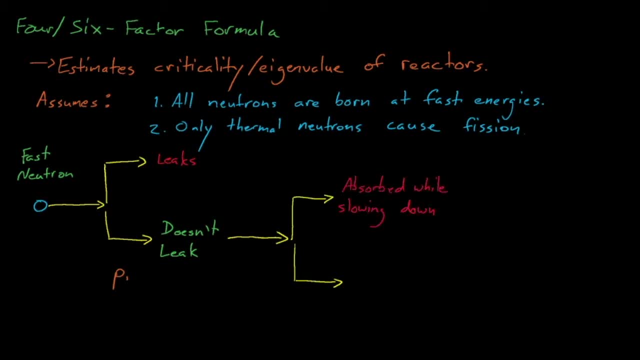 slowing down the thermal energies, which again removes it from the fission chain reaction, or it can survive the slowing down process and thermalize. Let's use p2 to describe the probability that this neutron survives and thermalizes. Once our neutron thermalizes, it can either leak or it could not leak, and we'll assume that p3 is a probability that our thermal neutron can survive. 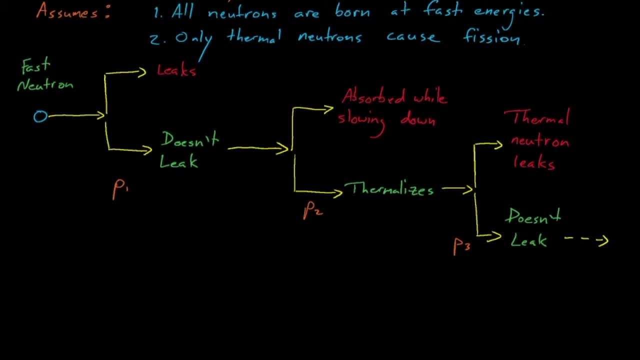 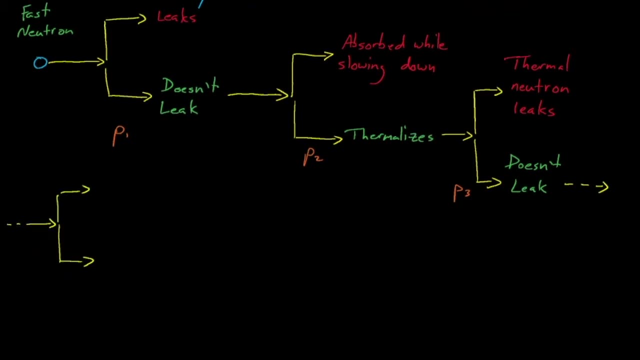 thermal neutron doesn't leak. Since we know that our neutron doesn't leak, we know that it must be absorbed by something in the reactor. The neutron can either be absorbed by structural materials, such as by the pressure vessel or the fuel clad, or it can be absorbed by the fuel. P4 is the 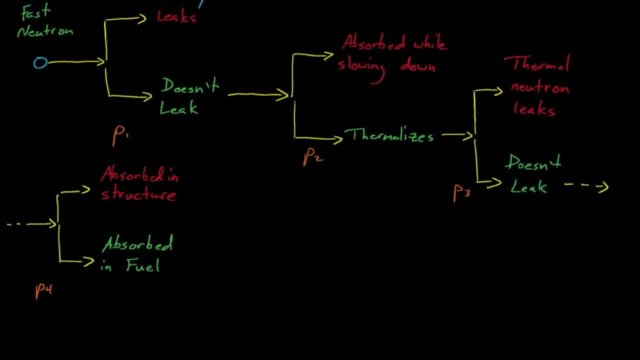 probability that the neutron is absorbed by the fuel. So now we know that our neutron has thermalized, hasn't leaked and has been absorbed by the fuel. And once it's absorbed, it can either result in a fission reaction and produce a fission neutron, or it can be absorbed by a parasitic. 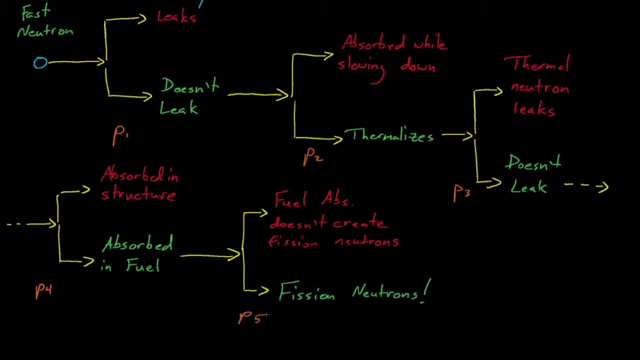 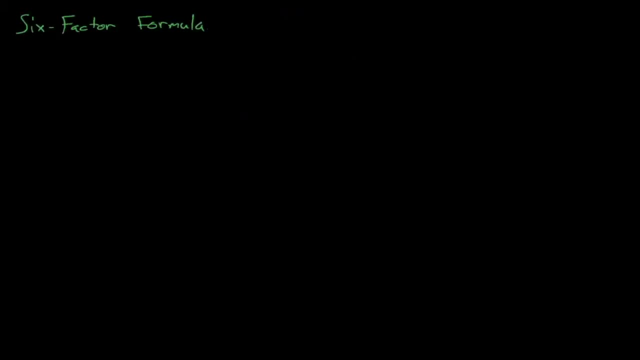 capture reaction. P5 is the probability that once our neutron is absorbed, that it will produce a fission neutron. So if we track our one neutron all the way through this event tree, we see that the probability that our neutron produces a fission neutron is equal to P1 times P2 times P3. 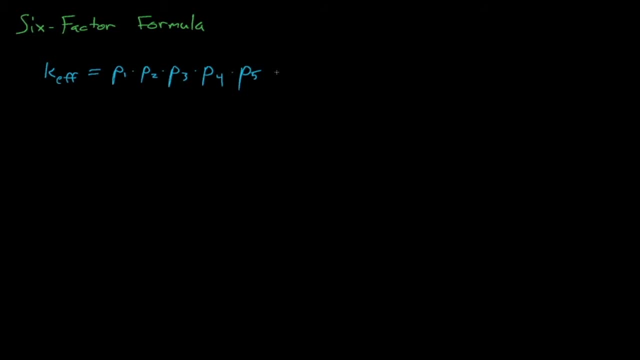 times P4 times P5.. In other words, our system's eigenvalue, which is the expected number of fission neutrons created by each fission neutron, is equal to the product of all of these probabilities. We'll also add this P6 term on the end of this expression, which corrects our 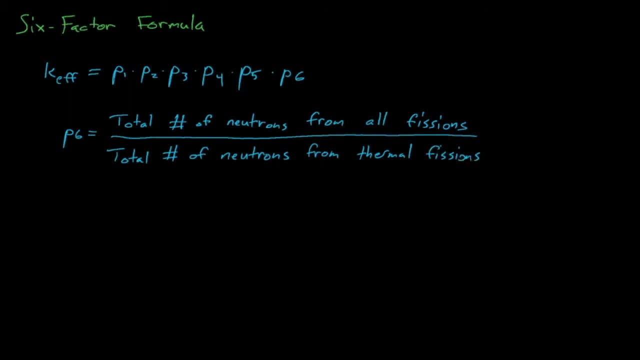 previous assumption that only thermal neutrons can induce fission reactions. P6 is the ratio of the number of fission neutrons that are created by fissions from neutrons of all energies so fast, plus thermal neutrons, divided by the number of fission neutrons produced by thermal neutron. 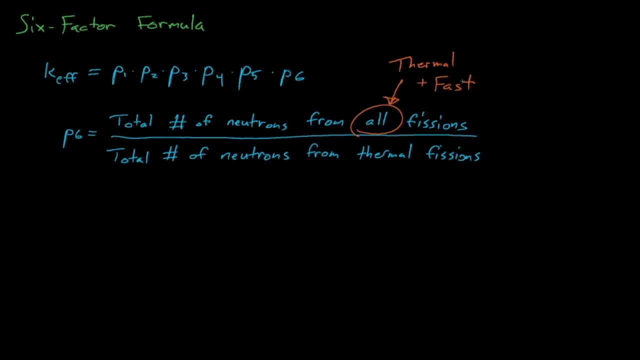 fission only. The combination of these two is the number of fission neutrons that are created by P6 probabilities is known as the six-factor formula, and it allows us to estimate the eigenvalue K effective for our system. These six factors describe some of the key reactor. 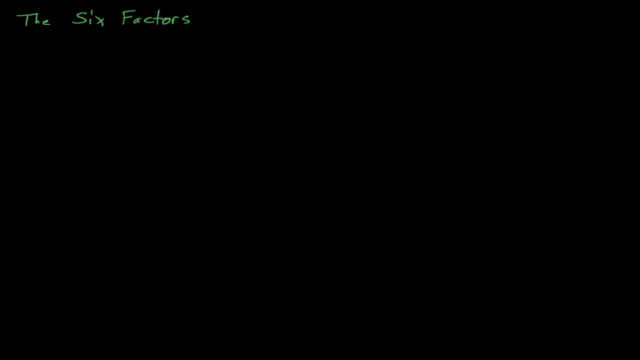 physics properties for our nuclear reactor and they actually have more descriptive names than P1, P2, P3, etc. P1,, which is a probability that fast neutrons don't leak, is represented by this P- not leakage fast. P2, which is the fraction of fast neutrons, 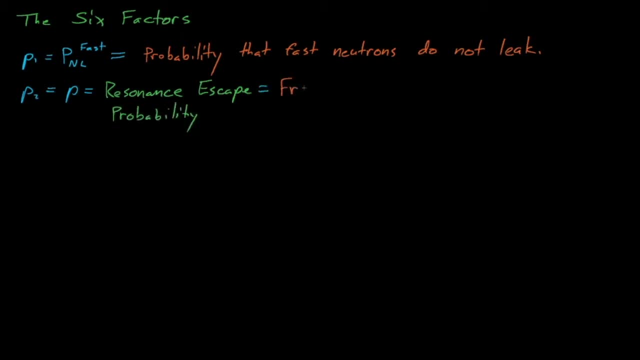 that successfully slow down to thermal energies is known as the resonance escape probability, and it's represented by the symbol P. P3,, which is the probability that thermal neutrons don't leak, is represented by this P not leak- thermal P4 is a probability that a thermal neutron that 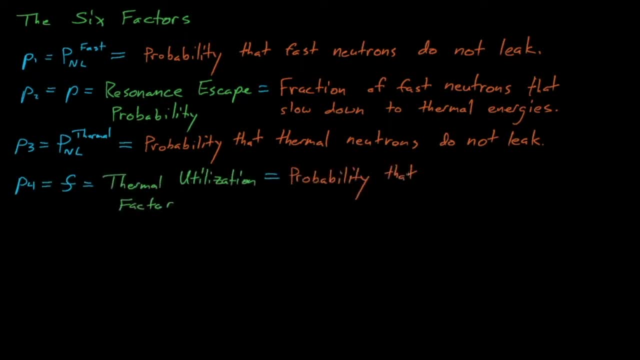 is absorbed will be absorbed by fuel, which is known as the thermal utilization factor F. The thermal utilization factor can be calculated by taking the inner product of the fuel absorption rate divided by the fuel and non-fuel neutron absorption rates. This ratio is also 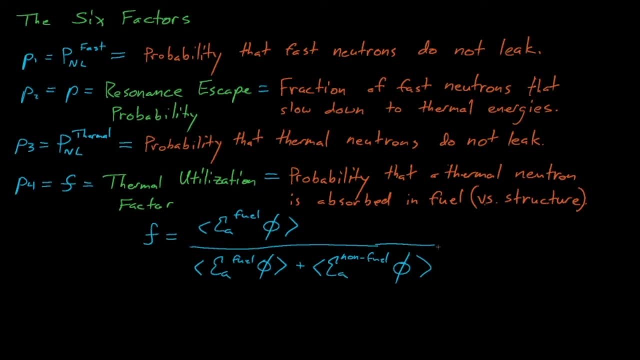 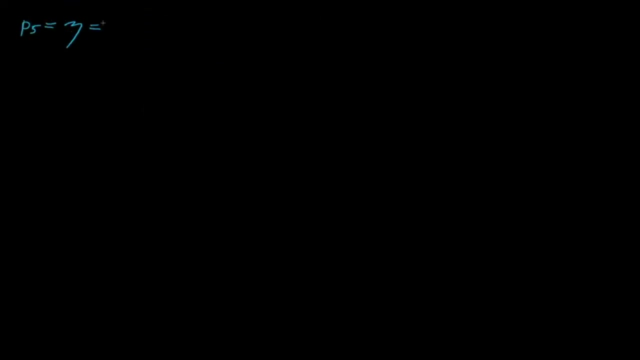 roughly equal to the ratio of the fuel absorption cross-section to the overall. so fuel plus moderator plus structure neutron absorption cross-section. We'll revisit this thermal utilization factor again near the end of the course when we discuss homogenization. P5 is the expected number of fission neutrons that are emitted per thermal neutron absorption. 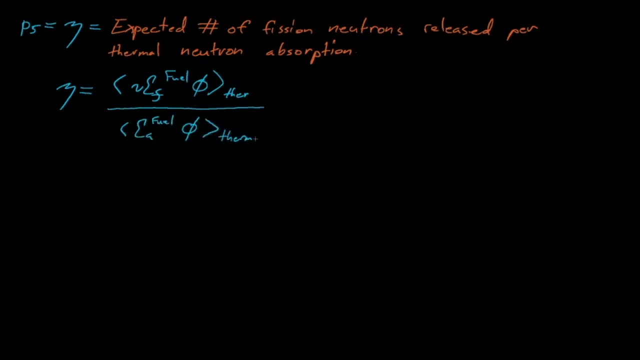 in the fuel, which is the number of fission neutrons emitted per thermal neutron absorption in the fuel. really just the value of eta for thermal energy neutrons in the fuel. Lastly, P6 is known as the fast fission factor and is described by this inner product ratio. 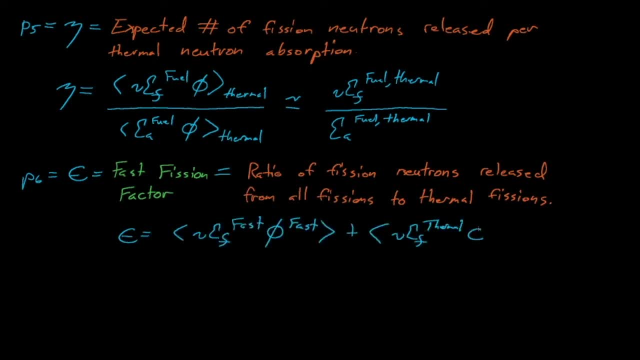 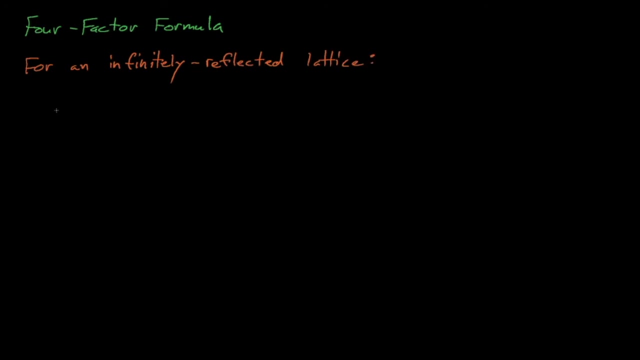 here, which is simply the ratio of fission neutrons released from all fissions to the number of fission neutrons released from thermal neutron-induced fission. only For an infinitely reflected system, the probability that our neutrons leak equals zero. In other words, if your system is infinitely large, then there is no way for neutrons to 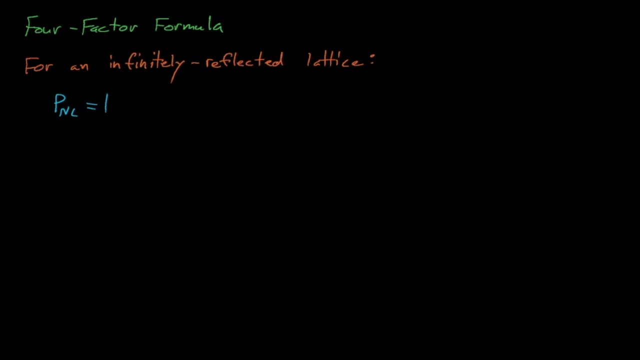 possibly escape. It's just like the thunderdome, except that one neutron enters and no neutrons leave. For this infinitely reflected case, our probability of not-leakage equals one, and our six-factor equation can be rephrased using only four of these probabilities. 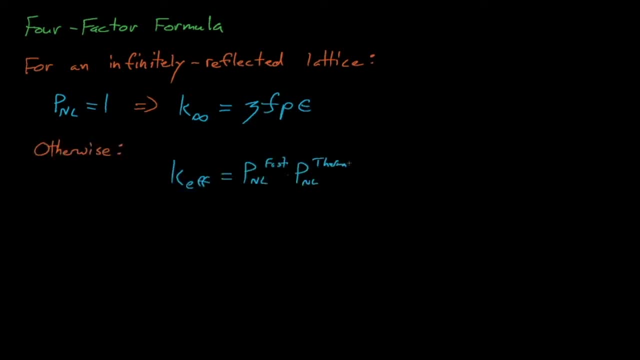 This is known as the four-factor formula. Since the four-factor formula describes the eigenvalue for an infinite system, this k-effective is instinctive. If we have a non-infinitely reflected system, then these leakage probabilities come back into play. Let's end our discussion today by discussing the typical values of an infinite system. 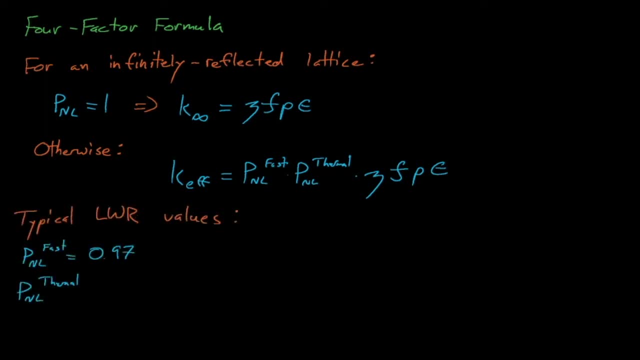 In general, the fast non-leakage probability is 0.97, and the thermal non-leakage probability is 0.99.. It makes sense that fast neutrons have a greater probability of leaking, since they have a longer mean-free path than thermal neutrons. 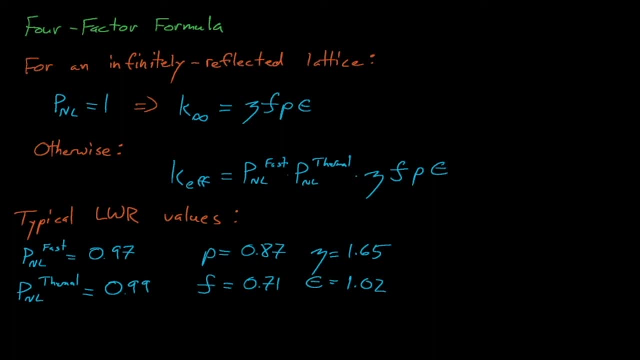 The resonance escape probability is around 0.87,. the thermal utilization factor is about 0.71.. Eta is around 0.1.. The thermal utilization factor is about 0.71.. Eta is around 1.65.. 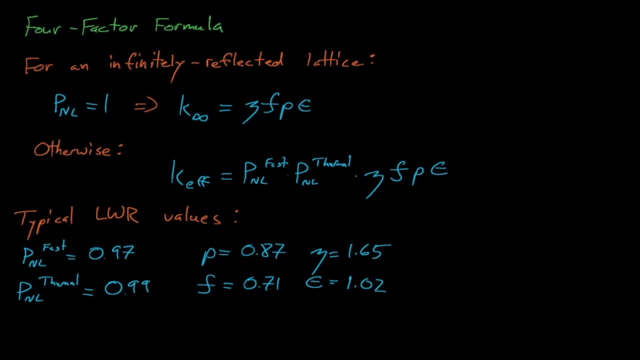 And the fast fission factor is about 1.02,, which means that roughly 2% of all fission neutrons are generated by fast fission. All in all, this means that our reactor's k-infinity is around 1.04, and that k-effective 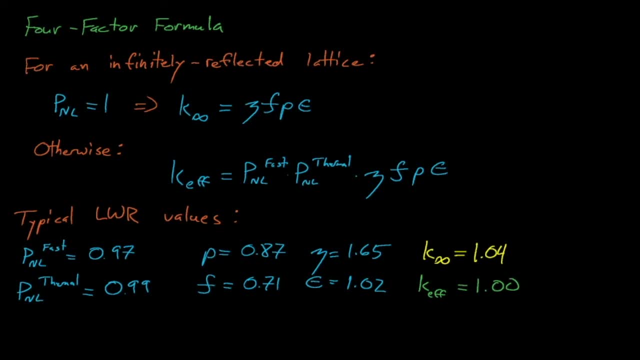 is a happy critical value of 1.00.. As a teaching tool, these six-factor parameters can illustrate how one might try to optimize a reactor design. If, for example, we sought to increase the eigenvalue of a reactor, we would have to 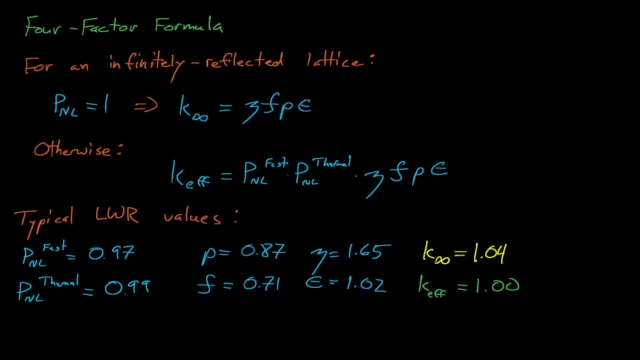 use the non-leakage probability. If, for example, we sought to increase the eigenvalue of a reactor, we would have to use the non-leakage probability. If we wanted to increase the eigenvalue of a conventional thermal reactor, we could either. 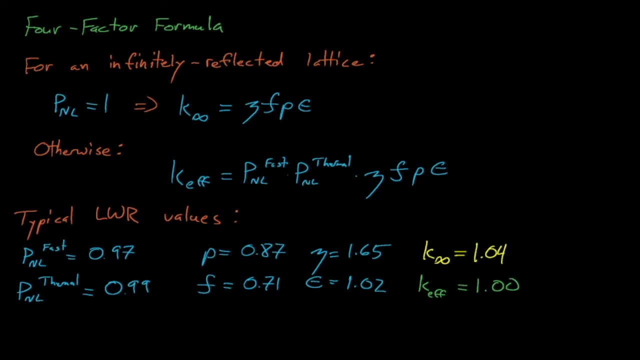 reduce the probability that fast or thermal neutrons will leak. we could reduce the number of neutrons that are absorbed, while slowing down to thermal energies. we could reduce the number of thermal neutrons that are absorbed in non-fuel materials. we could choose a better 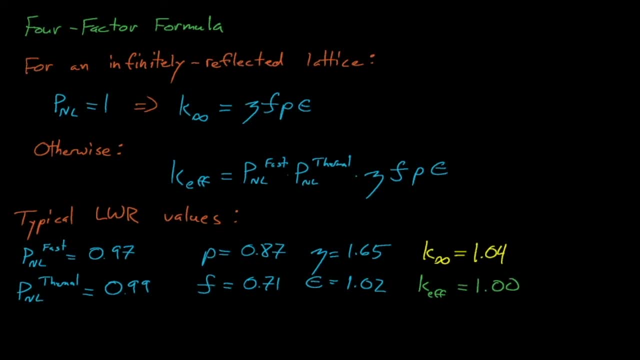 fuel material that releases more fission neutrons per thermal neutron absorption. or we could add a little extra oomph by getting some fast neutrons to cause fissions. This concludes our discussion of the four- and six-factor formulas. We may use these formulas to estimate the criticality of some simple systems, but really